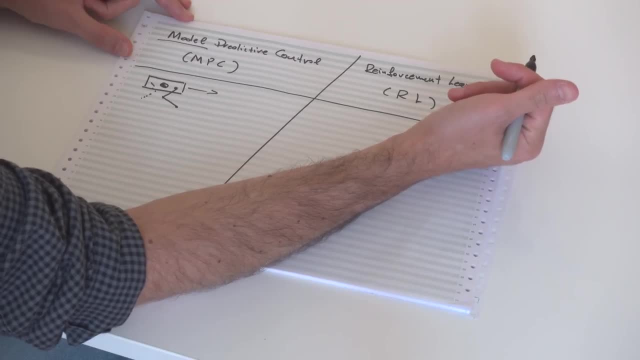 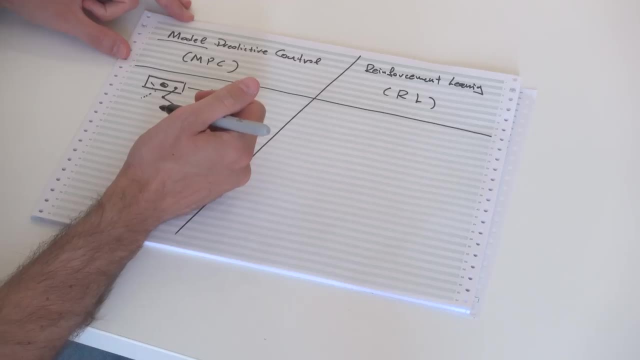 Three degrees of freedom. it means that it has three ways in which it can move right. It has three joints that, in most cases, are actuated by three motors. Now, each degree of freedom is one variable that we need to control And for the entire system, if we consider a robot with four legs, three degrees of freedom per leg. 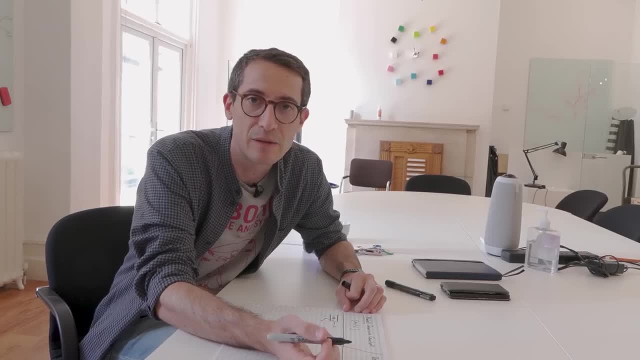 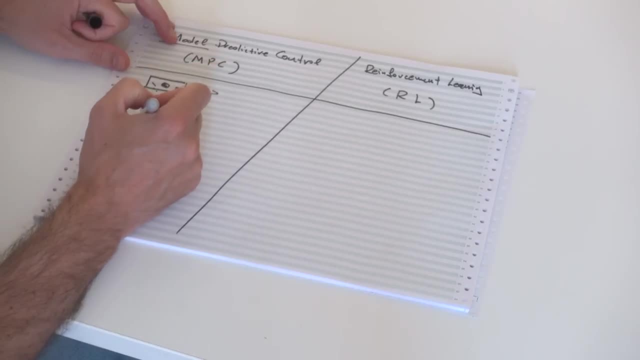 then we have twelve degrees of freedom for the joints, and then we have six more degrees of freedom about where the base position is with respect to the world. Now we model what each joint needs to do, And one way to go about this is to model that as a polynomial. 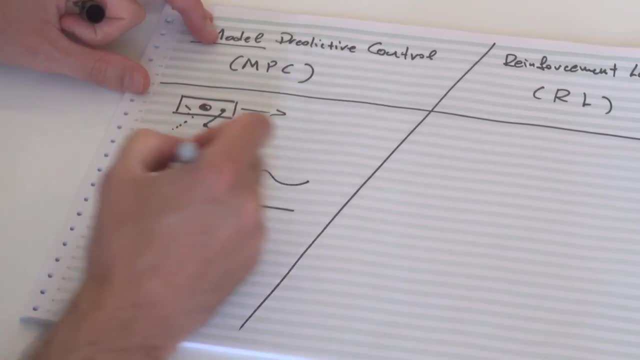 A polynomial would be a way of representing action, A curve, let's say against time, And be that Q be the position of one joint. In model predictive control, we would have a set of polynomials that would orchestrate how the robot moves. 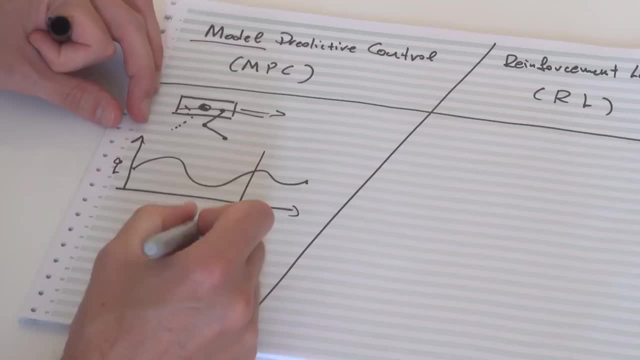 And then we would look at a time horizon, let's say capital T, And then forward, simulate the system, see what it does in the environment that it navigates, And then, for example, play out T, H, which is the horizon. 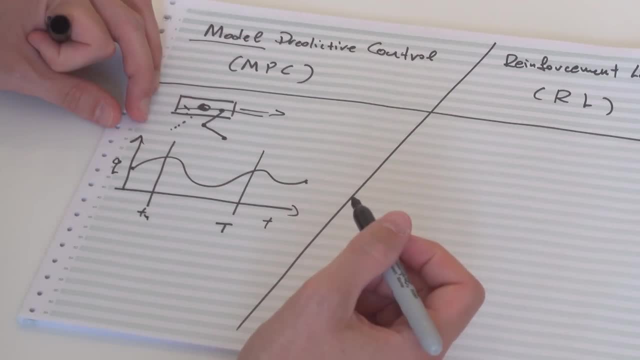 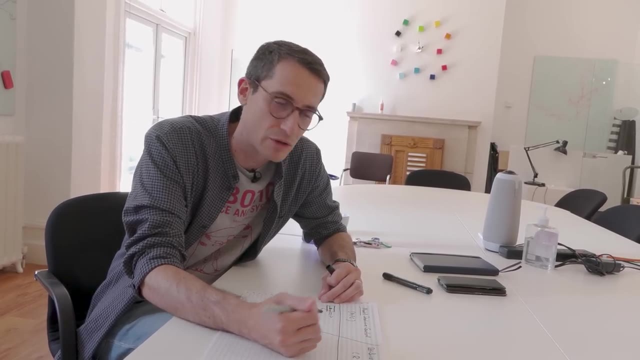 We can loop through that and repeat that multiple times And as time flows we sort of command the robot to do what it might, And this helps us deal with things like sensory noise, actuation, noise estimation, uncertainty and so on. 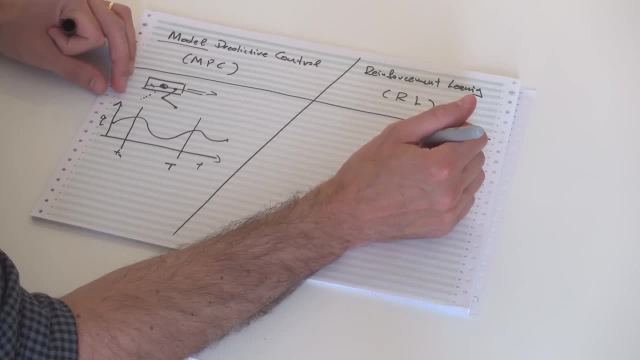 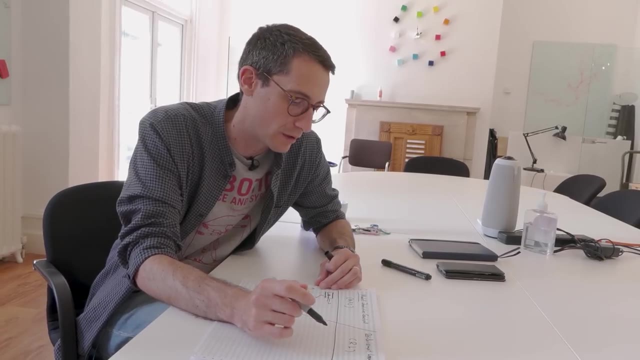 Drawbacks. We need to have good models of the system, And this is particularly difficult, especially if we're dealing with a system that is operating in a dynamic environment- is out in the world. You have things like wear and tear of motors or of feet, or actuators themselves. 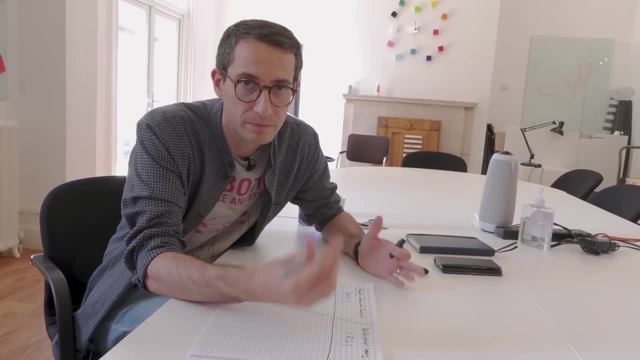 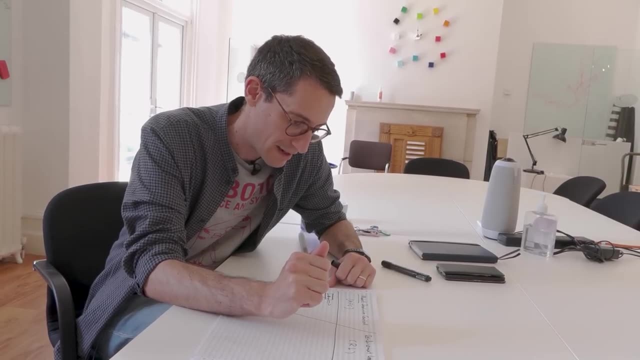 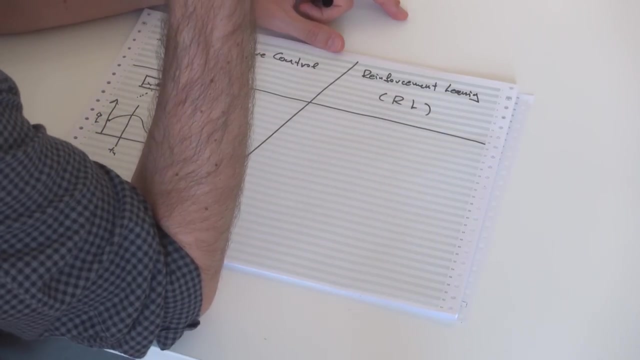 You have vibrations from making and breaking contact. You make and break contact all the time, which is an added complication. So this is the kind of analytical approach, the sort of more control-heavy approach. Now, on the other side we have a sort of- I think it's fair to say- more recent development on the machine learning side of control. 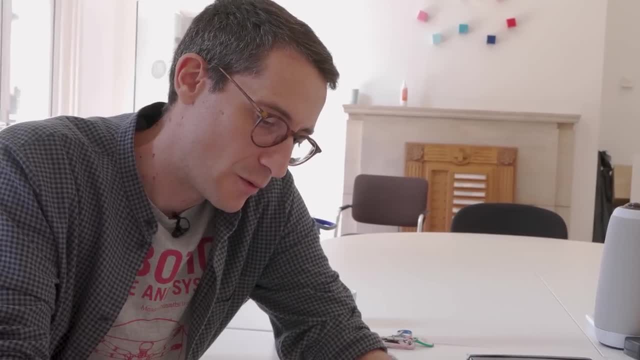 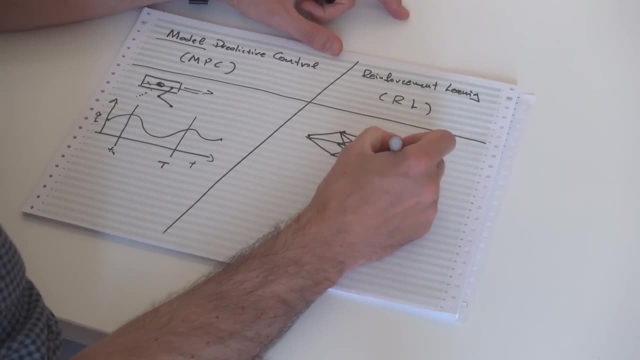 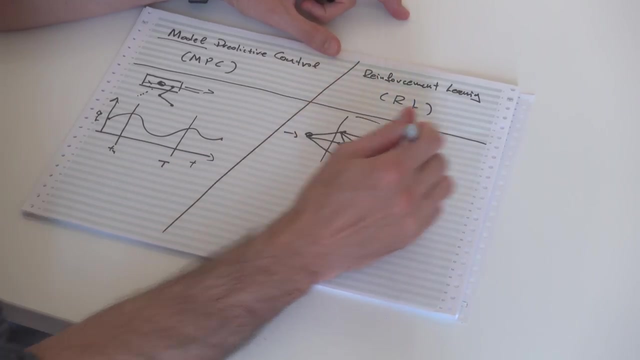 Where we train a neural network, as everyone these days. The idea here is that, this being a neural network, these are nodes, This is input and this is output. So we want to input the state of the system and get as output a vector of control inputs. 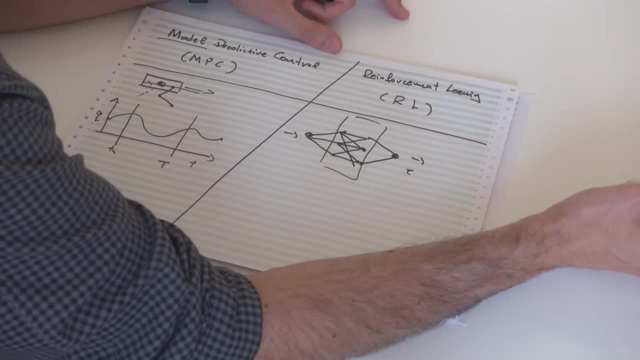 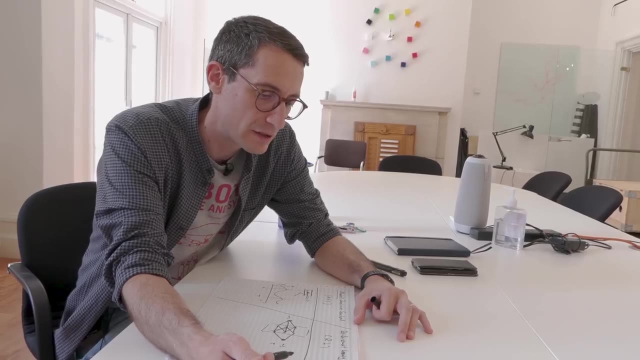 Be that the torque's position, desired position, desired velocities and so on- That accomplish a target that we set for the robot, for the system. In many cases, this would be being robust to external perturbations pushes Long story short. 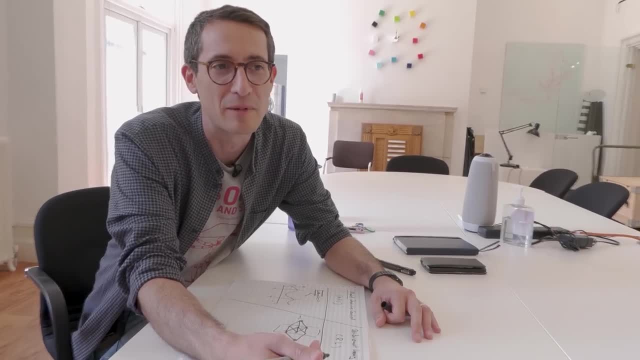 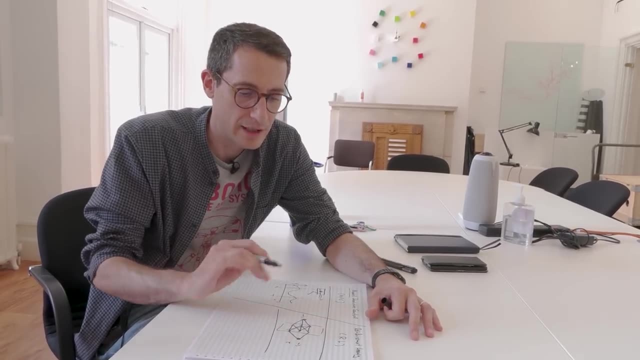 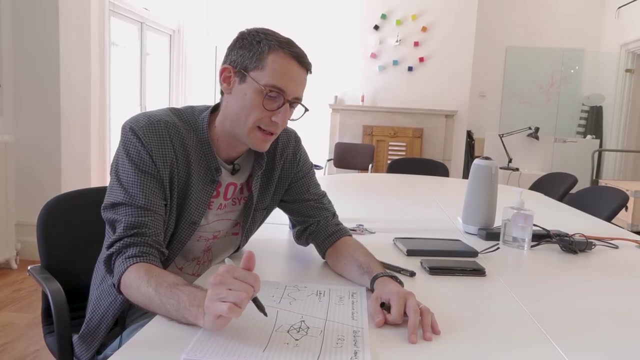 Long story short, the robot's not tumbling over and not falling and stepping on where it is supposed to step. The great benefit to that is that- okay, to start with, this operates with data. We would learn these controllers from data. 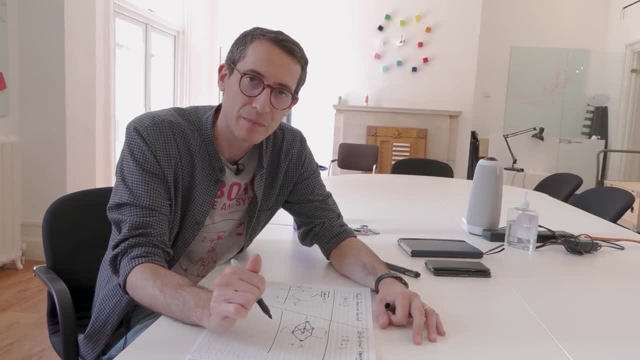 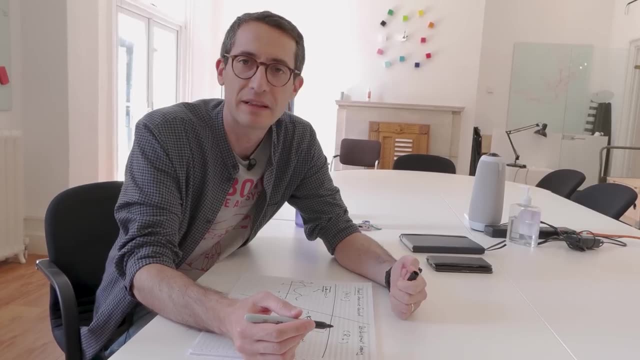 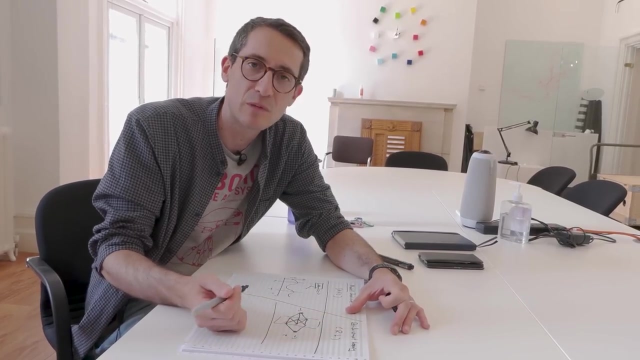 And the great benefit with that is that we can simulate examples, episodes that we learn from. So we can simulate the robot moving in an environment that we control And we can collect data of the robot performance and the controller performance in this simulation. We can leave that run sort of overnight, let's say. 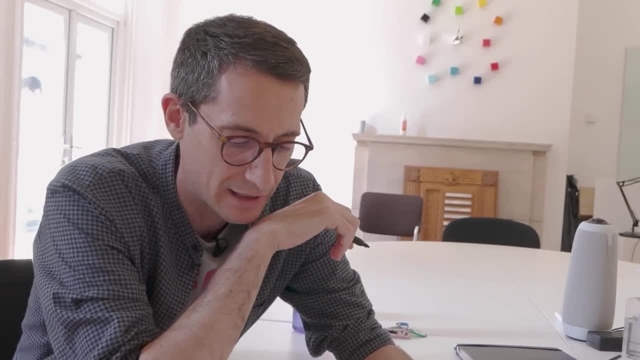 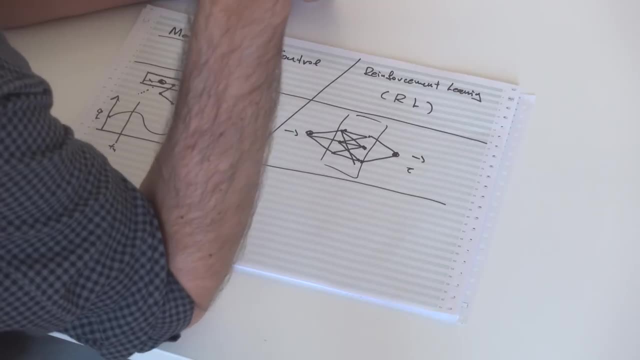 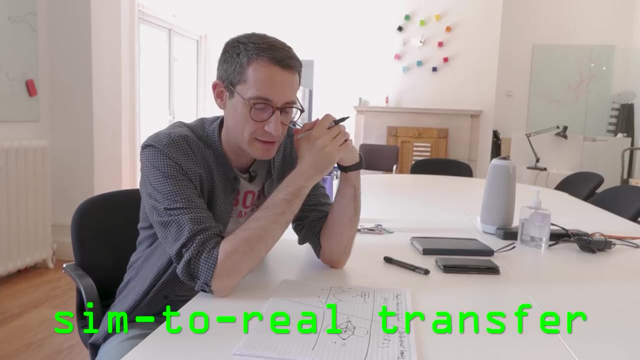 Or have a cluster that uses that, for that can do the simulations asynchronously And then we can use this corpus of data to learn very robust controllers. There is a complication when taking this from the simulation to the real robot. This is known as the sim-to-real transfer problem. 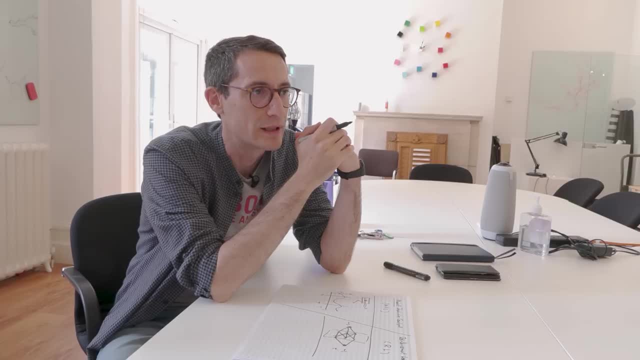 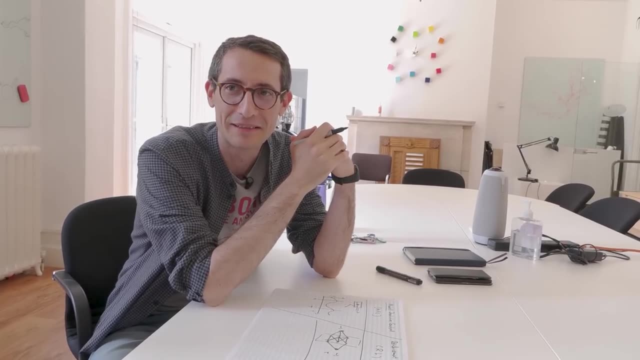 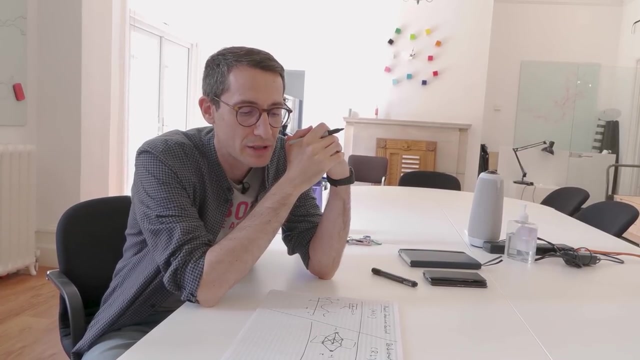 There are a couple of ways that we can work through that. One of it is double down on the machine learning approach And learn from data a model of how the system responds to our input, And the other approach is to actually bake that in into a controller learning. 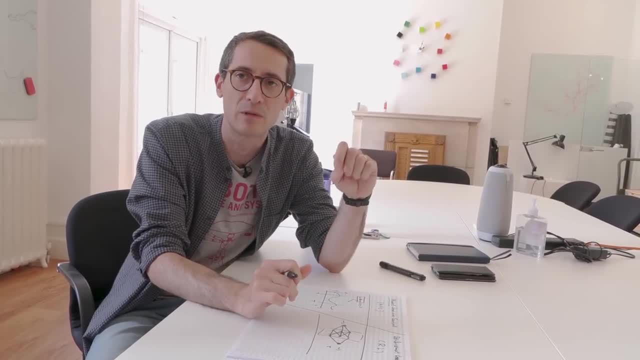 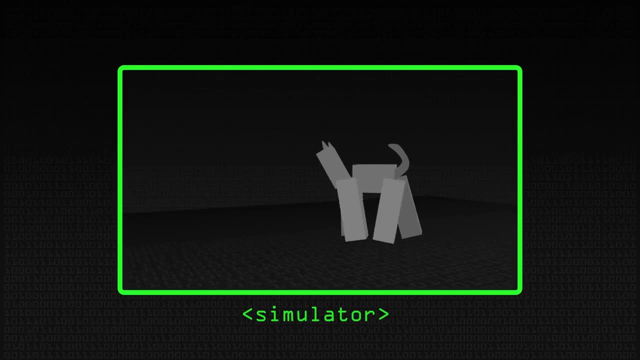 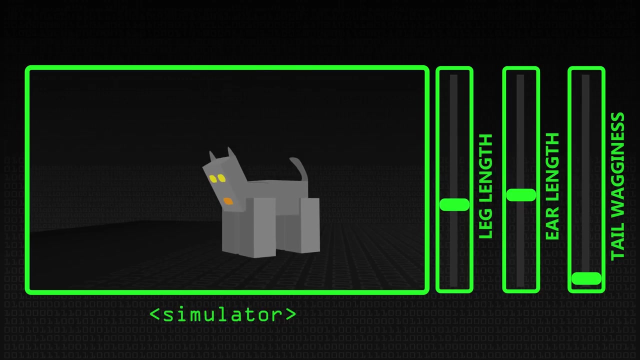 So instead of learning with one particular model in simulation, we have a range of models, that we think of it as a range, where we can sort of have knobs for each variable of the system. Imagine having a model of a quadruped where we can twist a knob and get longer legs. 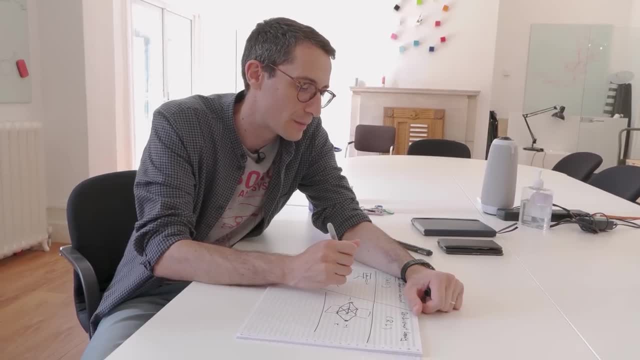 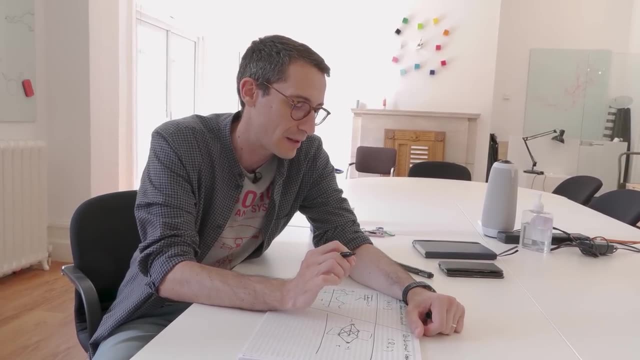 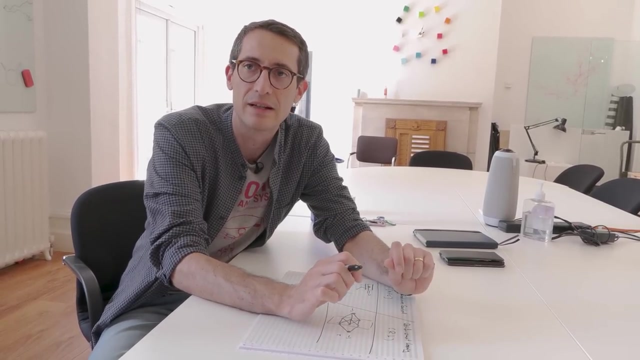 or shorter legs or larger bodies. We don't change the morphology, so we would not change the degrees of freedom. We would change the variables of the simulator itself. So by adding these variants we can make the controller robust against changes in that parameters. 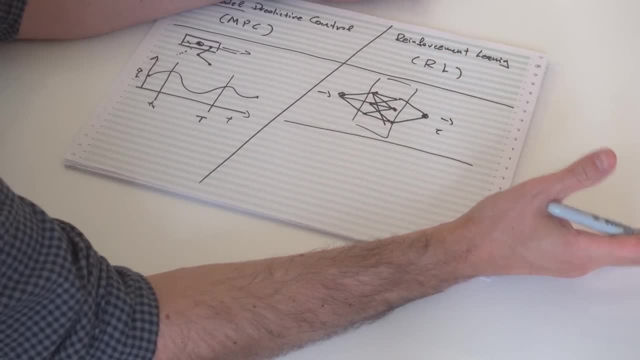 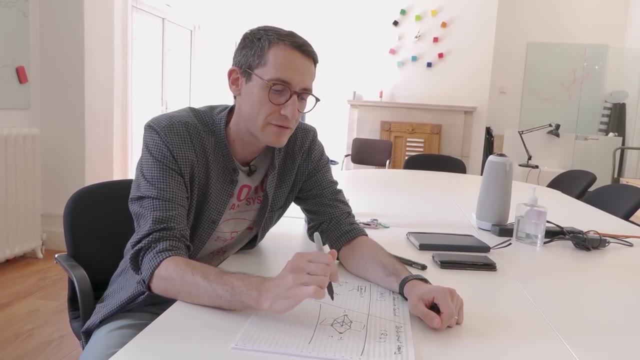 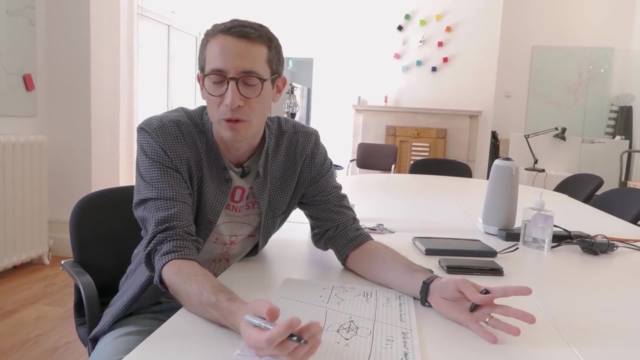 And these are the set of parameters that are hard to estimate from the real system and accurately approximate in the simulator. So we can make our controllers robust to variations of these parameters, which means that it can transfer to a somewhat different model, which is the model that it's not the model, it's the real system, right. 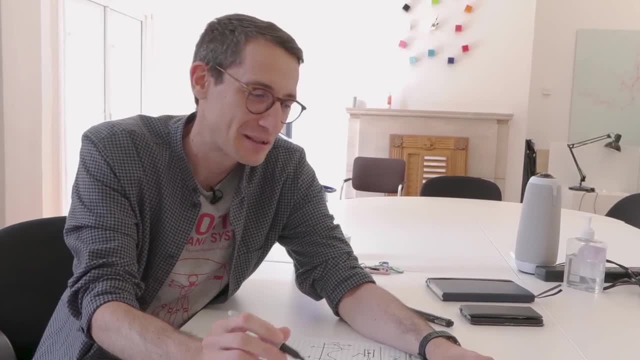 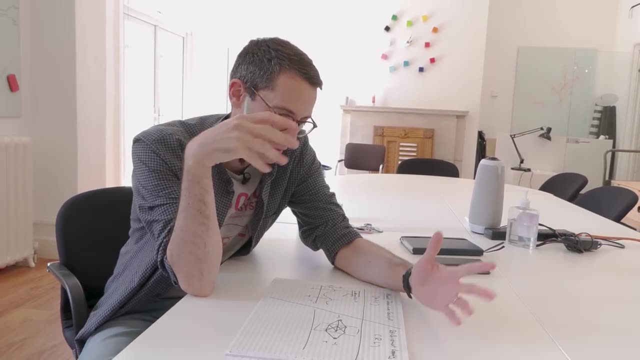 Okay, so can we see some of this? Is that possible? Absolutely yeah. We have one of our quadrupeds downstairs in the lab and we can show you what the robot does in the lab In walking over some of sort of our benchmark obstacles. 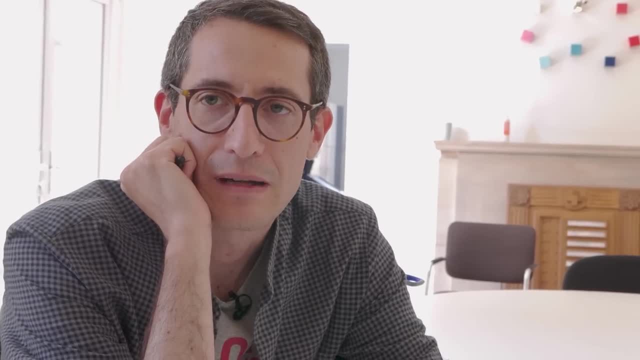 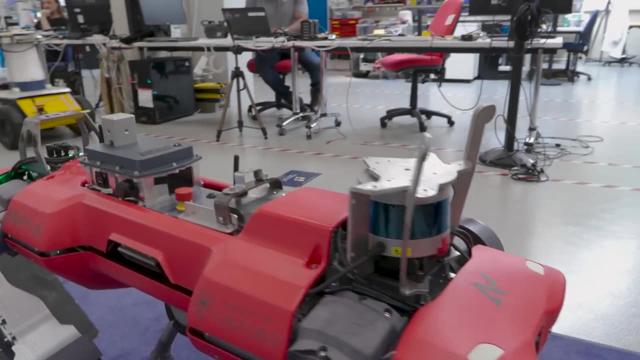 And we can also have a look at what the robot sees, how the robot models its surroundings and where it decides to step, and so on. So this is a quadruped robot, right? This is animal version C. Its name is Coyote. It's one of the robots in our lab. 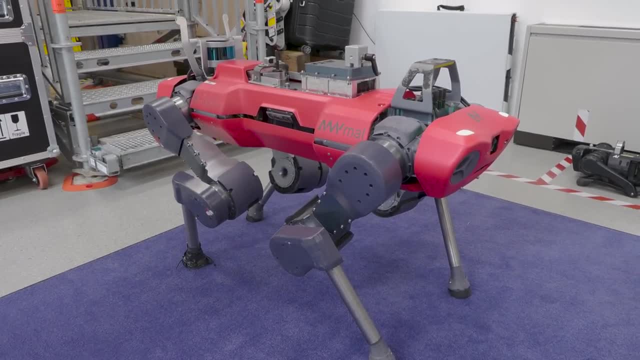 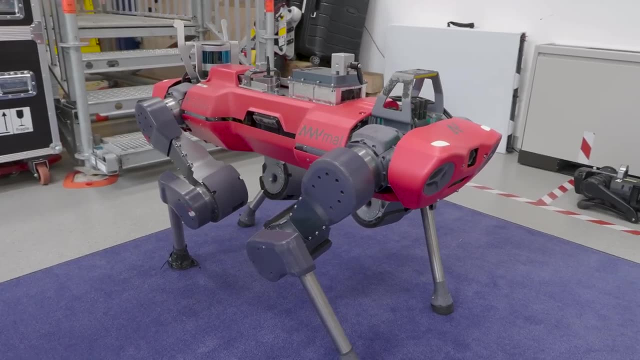 The research that we do here is we're looking into machine learning approaches to legged locomotion. This is quite different from traditional approaches that use, for example, model-based control or model predictive control. There is a kind of convergence in the fields at the moment. 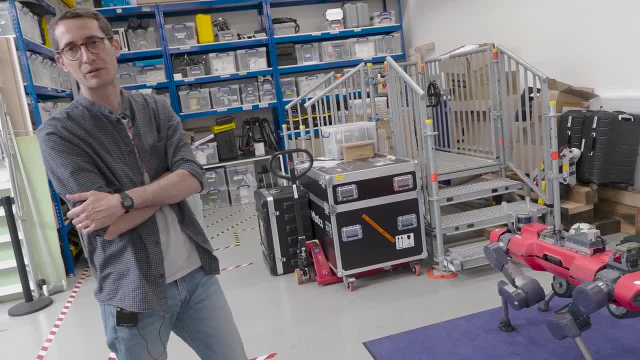 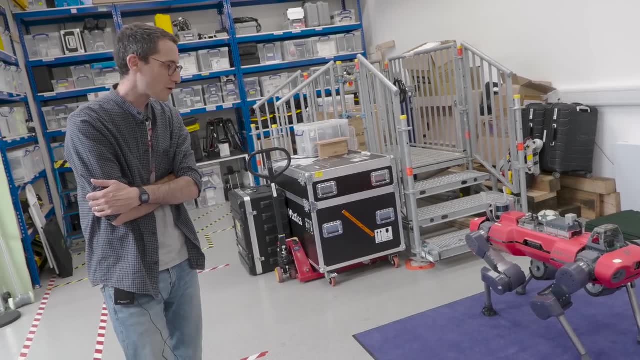 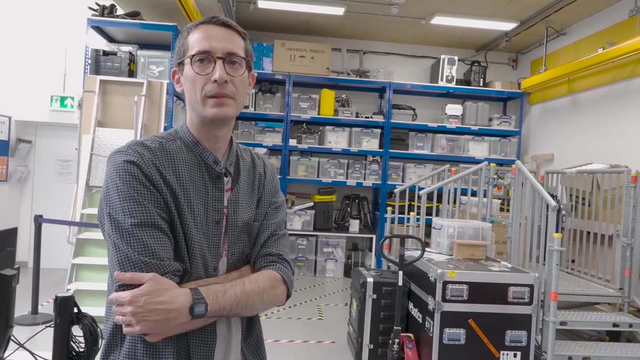 We are working and we're seeing a lot of approaches that combine model predictive controllers and learned aspects to these controllers. Now Sid here is going to demonstrate our RL-based learning controller right, This is a controller that has been trained in simulation, having a set of controls. 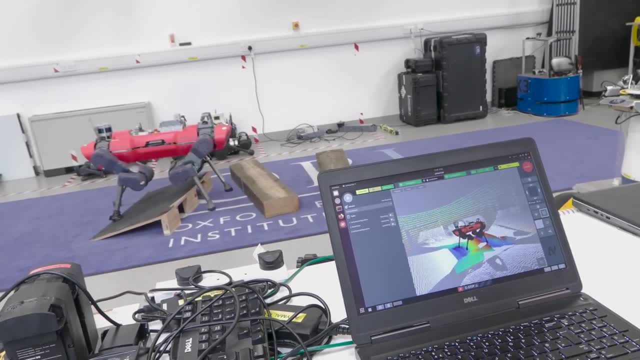 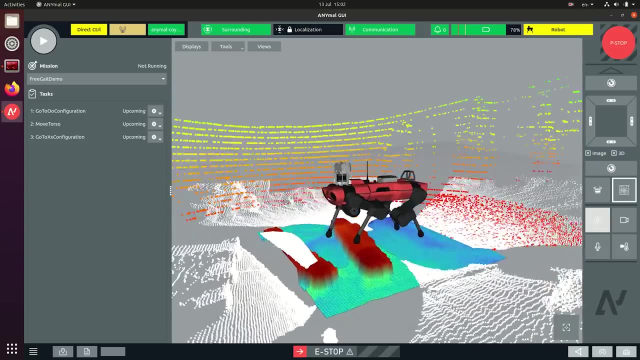 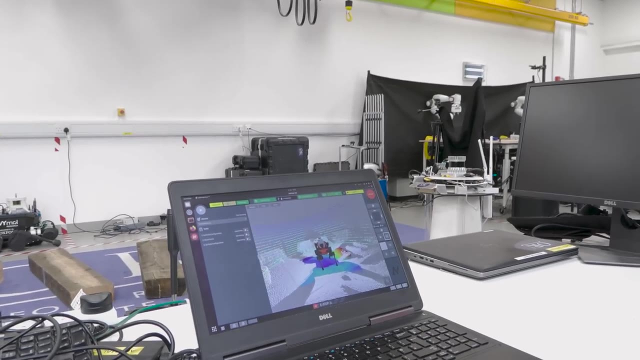 We have a set of examples shown to a neural network that learns to control the system, And after having it trained, then we can run it on the robot and evaluate its performance. So you've got a projection there that's kind of similar to where we're standing, isn't it? 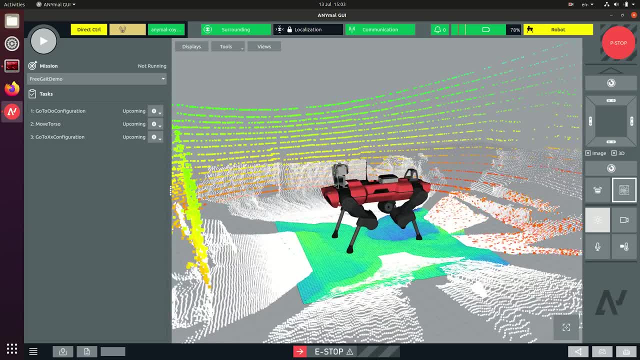 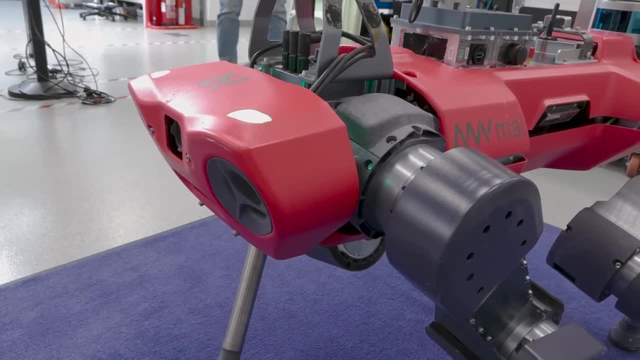 So what's going on there Exactly? So we can. These are the LiDAR returns from the LiDAR sensor that's there on the back of the robot And then on the robot. there are four depth sensors that are distributed around the body. 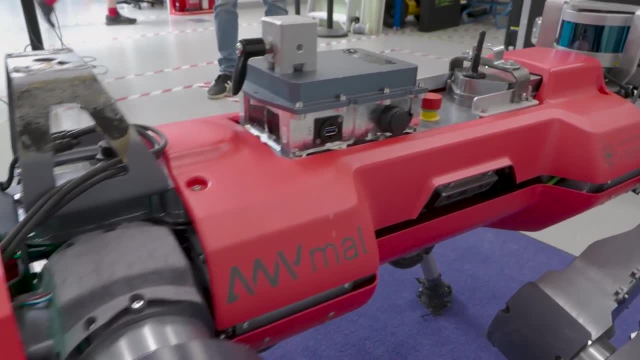 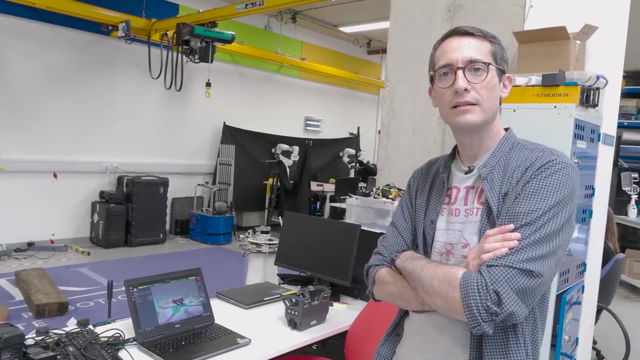 And this is the estimate of the system, of how the ground looks around its feet, And with that the controller can decide where to place its legs. This is an estimate, So there's still. The robot can still stumble and sort of place feet at the 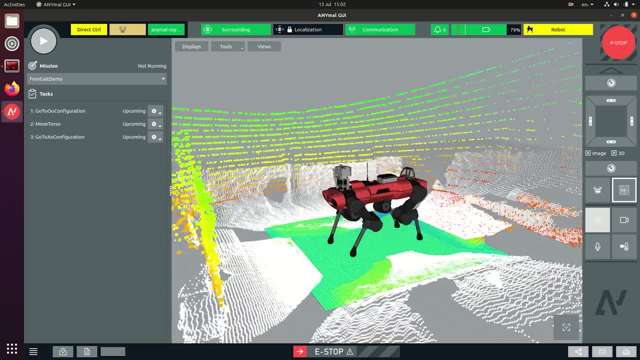 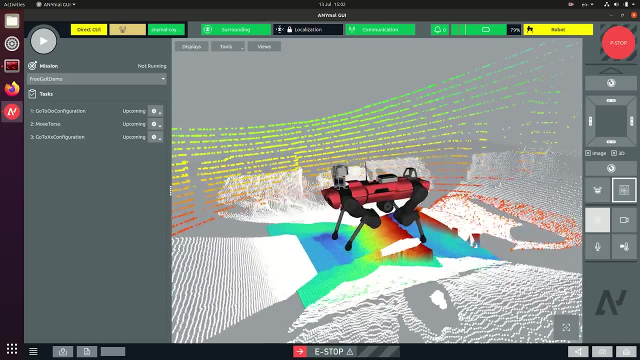 sort of a position where it can Sort of feel its way, almost. Yeah, The goal here is to have a controller that is also robust to slipping. That plank could be wet, it could be slippery, Yeah exactly, Or stumbling, and so on. 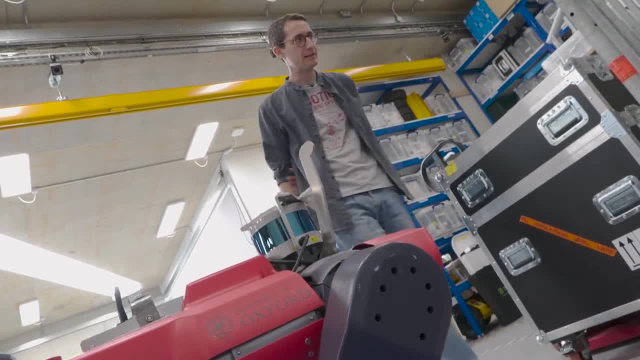 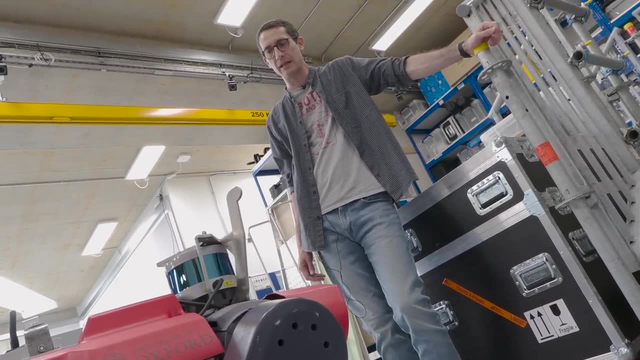 This is Animal in its version C. This is built by a company in Zurich that builds robots and we've been working with for quite some time now. That is a spin-off of the ETH University in Zurich. We talked about different methods of learning upstairs. 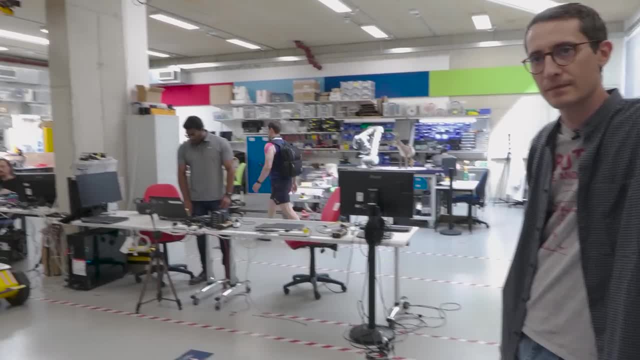 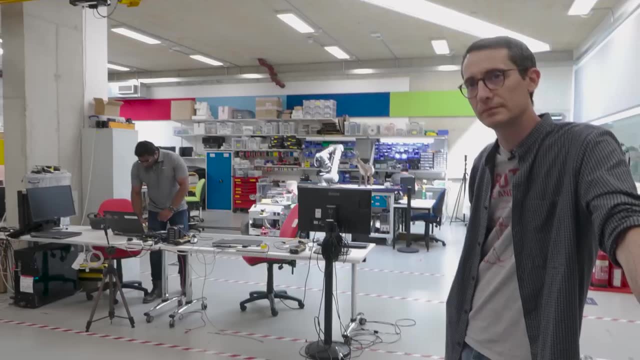 the reinforcement learning or the model bay. Where does that fit in with doing that then? Is that then You've not got a static kind of equation that you plug all those numbers into? it works differently, doesn't it? Yeah, exactly. 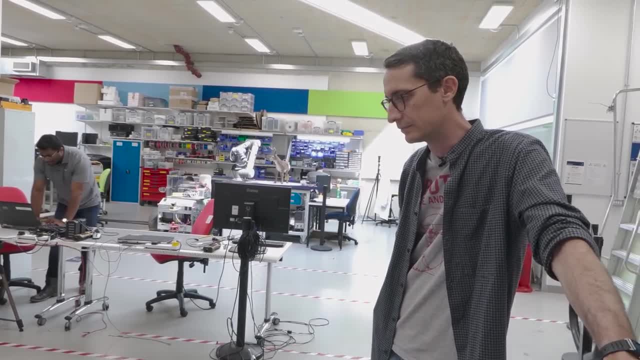 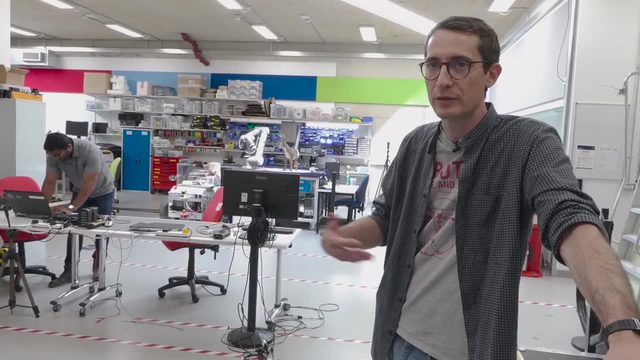 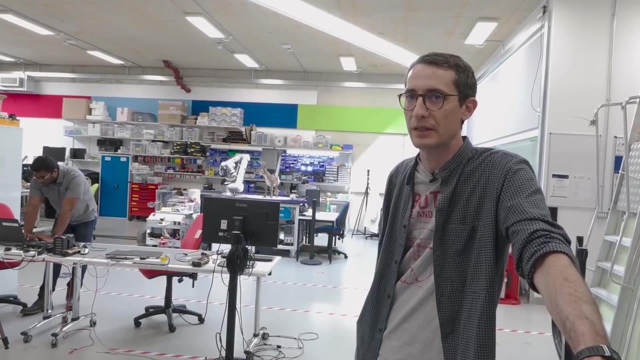 So this is a neural network that then online receives perception information from the joints and the torque sensors and the vision and depth sensors, and then decides where to place feet and how to orchestrate the motion of all the actuators in order to be able to coordinate the system. 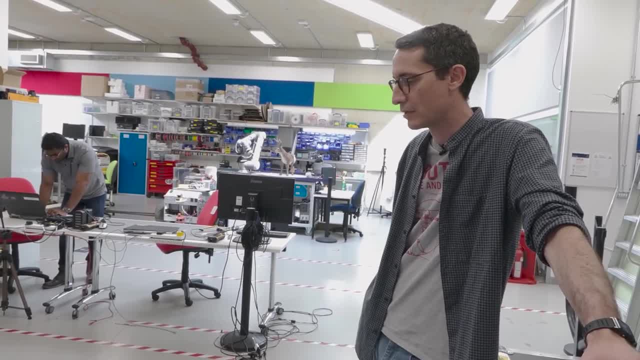 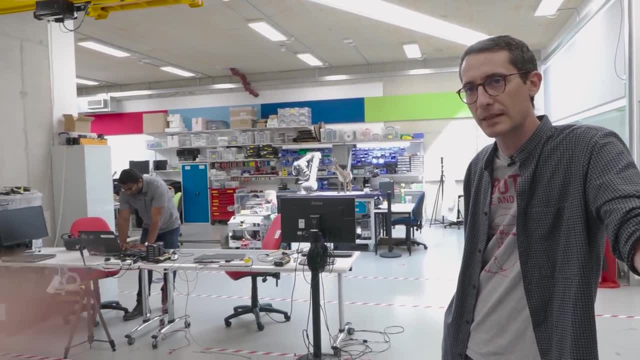 into walking over things and going up flights of steps and going down flights of steps and so on, And so is it learning as it goes. or is that then a It's already done the learning, and then you've applied that to the Yes in this particular controller, the learning has been done. 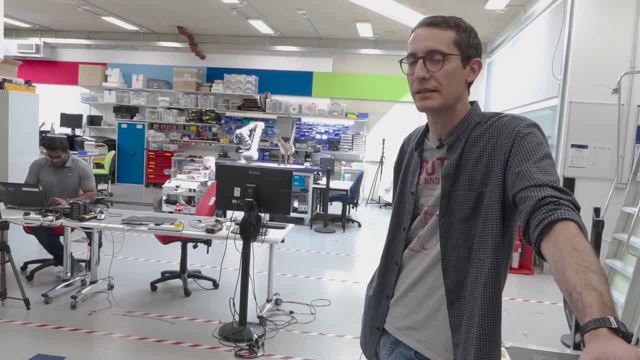 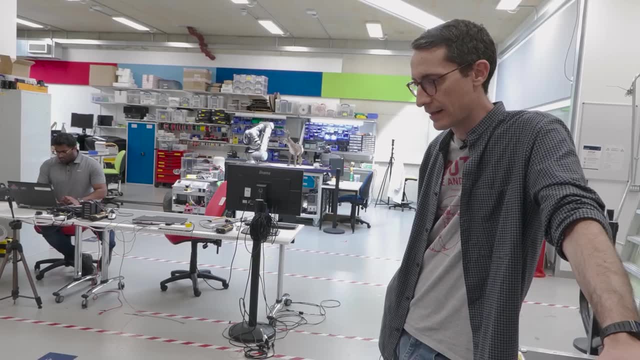 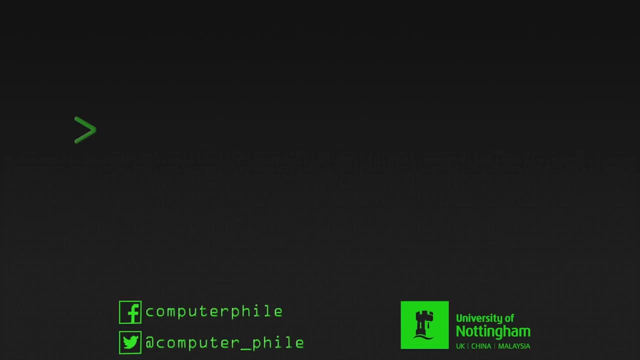 and it's not learning as it goes, but we're currently looking into approaches that we can distill some of the online experience of the robot and see how we can incorporate that into a sort of ongoing learning system. Right, so this is the signature here.